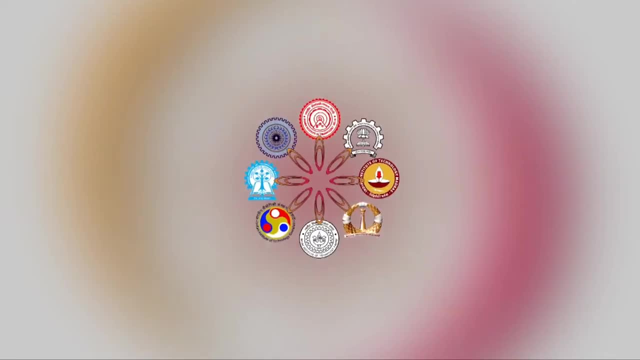 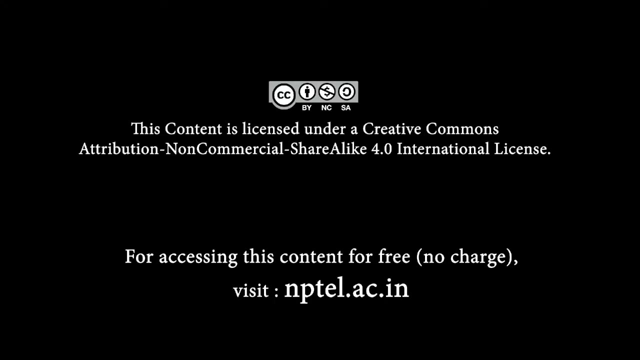 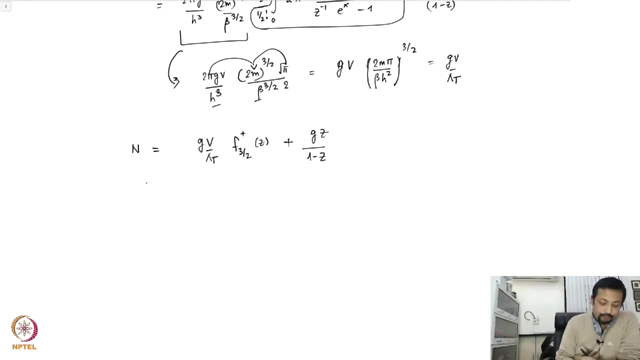 So now we have this expression for n, which is essentially g, v over lambda t, f of 3, half plus z, the plus, denoting that we are looking at a bosonic system: n, 0, z. So as usual, the fugacity has to be determined from this relation. but if you look at this function, f of m eta. 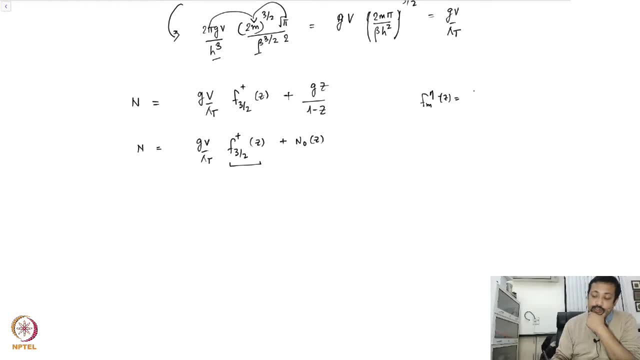 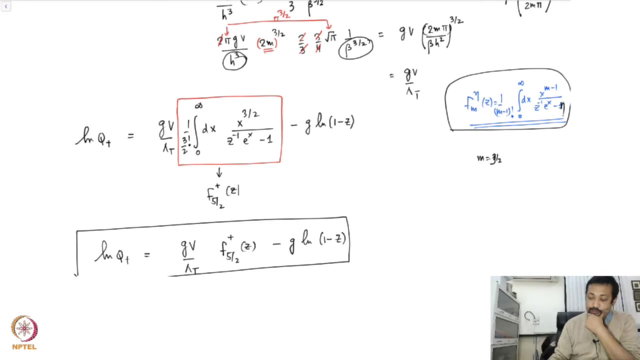 of z was 1 over m minus 1. factorial 0 to infinity d x. So x to the power m minus 1 z. inverse e to the power beta minus eta. I think we did make an error. while we sorry, this has to be minus of eta for specific eta. If it was plus then 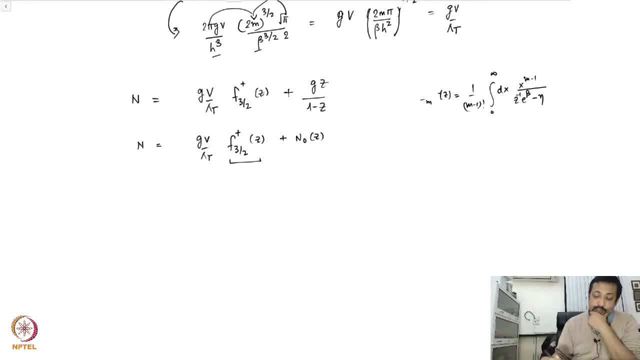 I know that this is just going to be f: m plus of z is just going to be minus of 1 beta epsilon. Ah, terribly sorry for the mistake. this has to be e to the power x minus 1.. Now, this is a very complicated function and usually its representation in terms of simple functions. 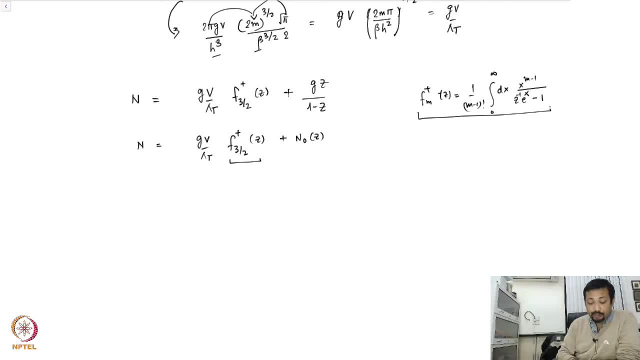 are not possible. but we do know the high temperature expansion of this, The high temperature expansion of f m. so temperature expansion gives us f m plus of z was 1 over m minus 1. factorial. this was already taken care of. it was simply sum over k equal to 1 to infinity z to the power k. 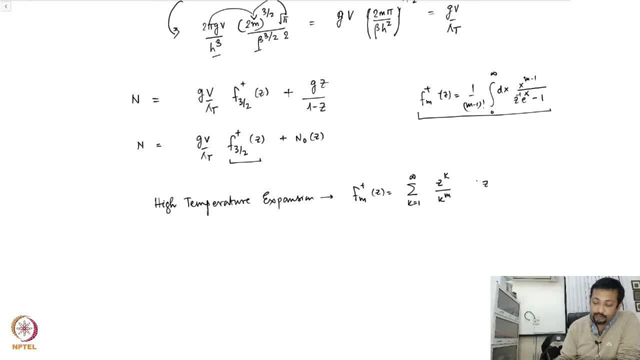 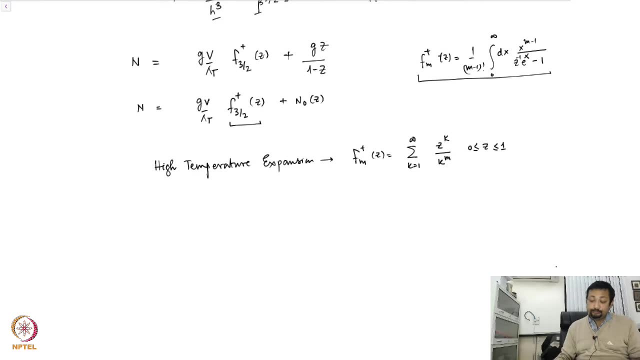 to the power m for z greater than equal to 0, less than equal to 1.. One should note that if I set z equal to 1, so f m plus of z equal to 1 becomes sum over k equal to 1 to infinity. 1 over k to the power m minus 1 factorial. 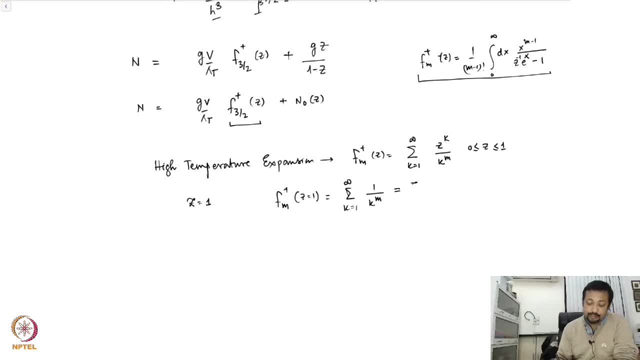 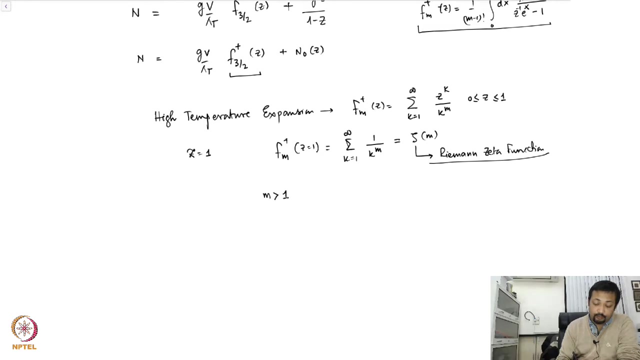 And this is zeta of m, where the zeta function is the Riemann zeta function, The series converges for m greater than 1. And f plus m of z tends to infinity. for m less than 1, as z tends to 1.. 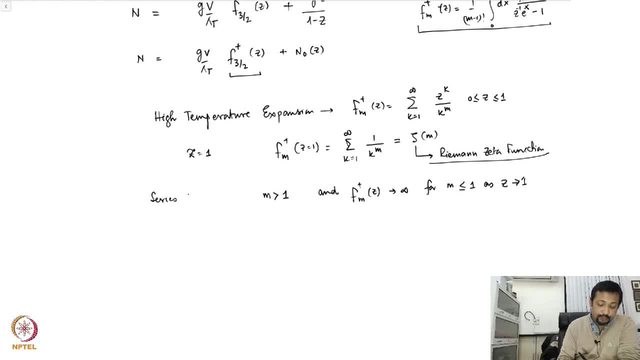 So series converges for m greater than 1, and f plus m of z goes to infinity if m is less than equal to 1, as z tends to 1.. On the other hand, f plus m of z is finite for all m greater than 1 and for z greater. 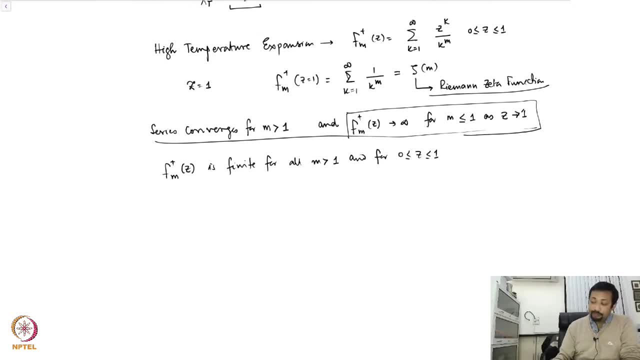 than equal to 0, less than equal to 1.. So, coming back to this, then I have coming back to this expression, for the particle number is f of 3, half plus of z plus g, z, 1 minus z. The first term that you see over here is: 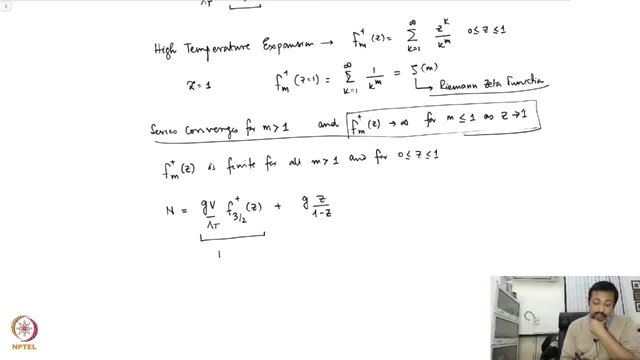 the term is the number of particles which is contained in the excited states and this is the number of particles which are contained in the ground state, n equal to 0.. So this is the term. the first term is the term which is contained, the which essentially represents. 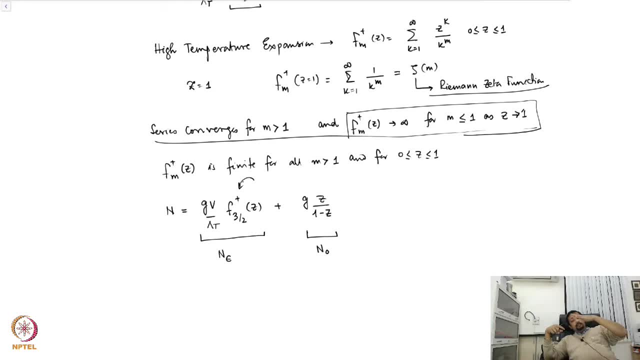 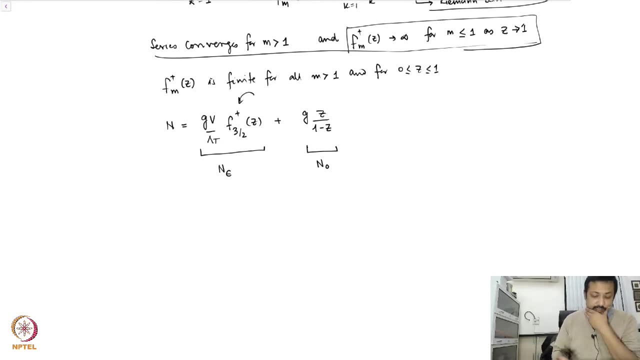 the particles contained in the states other than the ground state. but now we have clearly seen that. So this term is limited by this function. right, and for a Bose gas, I know that the maximum value of z can happen. there is a limit on values of z, that is, z can be greater than. 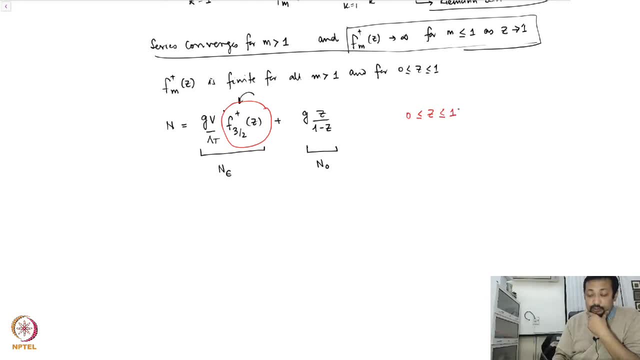 equal to 0 or it must be less than equal to 1.. So clearly, when z approaches 1, then this part, the first term. We will write down this as n epsilon maximum. there is a maximum number of particles which you can accommodate in this excited states, and that number is given by G v over lambda. 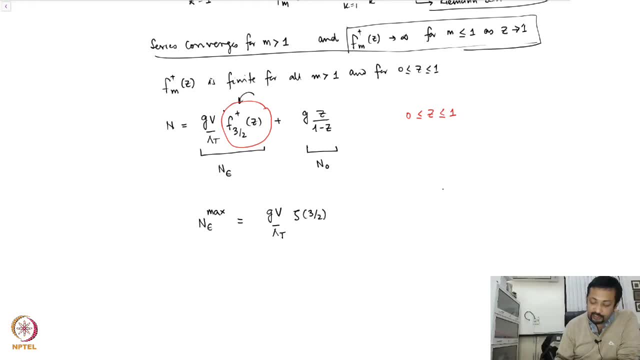 t, zeta 3 half, where zeta 3 half is approximately 2 point 612.. Okay Now, this is a very important inference. You see from the expression for the total number of particles in your system that you can accommodate only a certain number of particles in the. 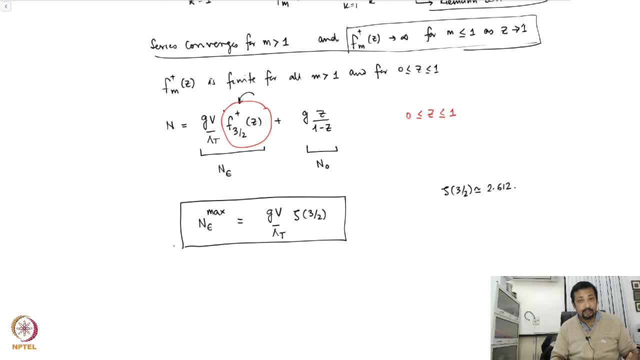 excited stage. There is a limit upper bound on that. So if you keep on adding particles to the system, you are going to hit this limit. and then, if you keep on adding more and more particles, where do they go? They go to the ground state, and that is when your condensation 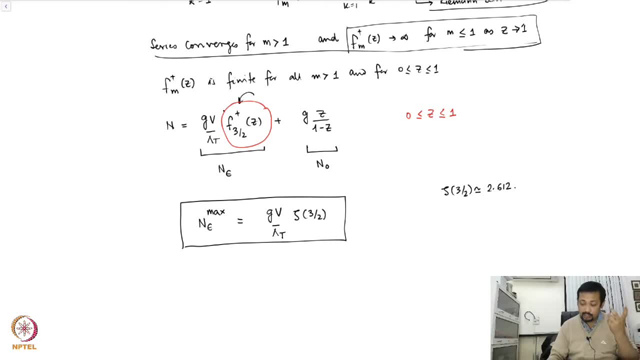 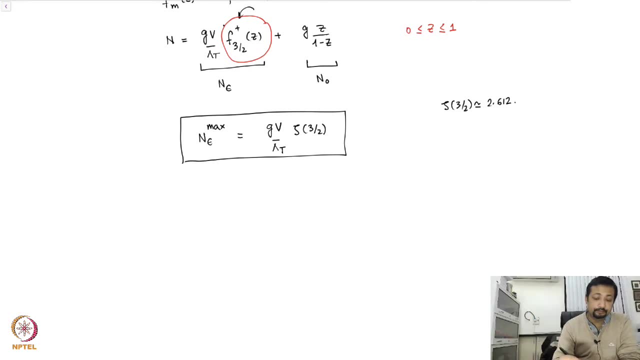 starts to appear- Sorry, not. the condensation starts to happen and the condensate starts to appear. This goes as V? t to the power. three. half, On the other hand, not well, let us. So the second term. this is the term, and 0 can be ignored if z is very. 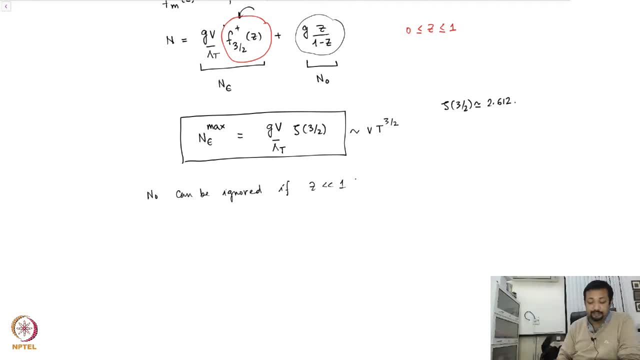 very less than 1.. So if you are not hitting the limit of z to 1.. On the other hand, if n, the total particle number, is dominated by the number of particles in the ground state, so that you have n, z is approximately this: you see what happens to z. This implies that 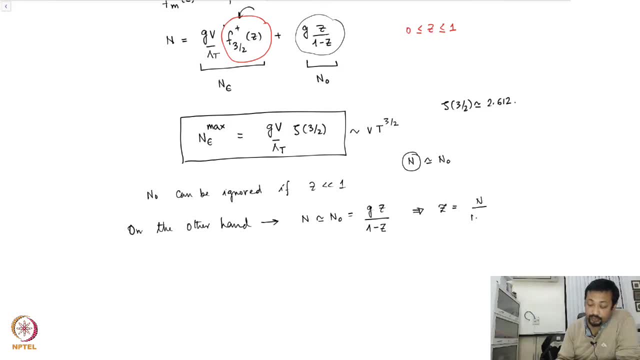 z is approximately n over n plus, not approximately, but exactly n By n plus g. g is a tiny number compared to n, which is 10 to the power 23 typically, and therefore, you see, this value is 1.. So, whenever this condition is satisfied, that 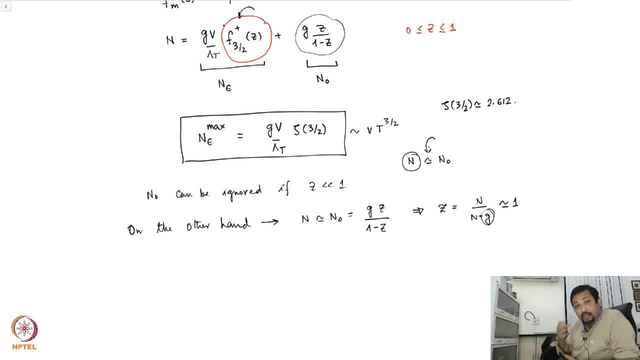 you actually see that the number of particles in the ground state start dominating the total number of particles in the system. So most of the particles have gone into the ground state. then you have actually hit the limit z equal to 1.. So in the thermodynamic limit, 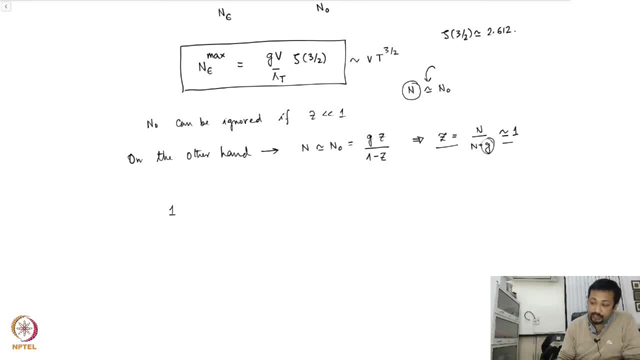 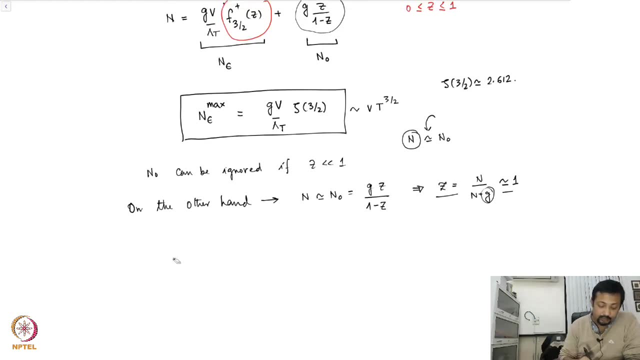 we rewrite this equation which we had over here and a little up, So we had the expression: n was equal to n epsilon plus n, 0,. we rewrite this equation as: 1 is equal to n epsilon over n, plus n, 0 over n. 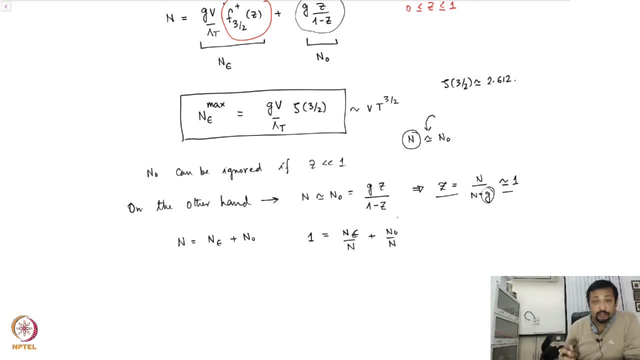 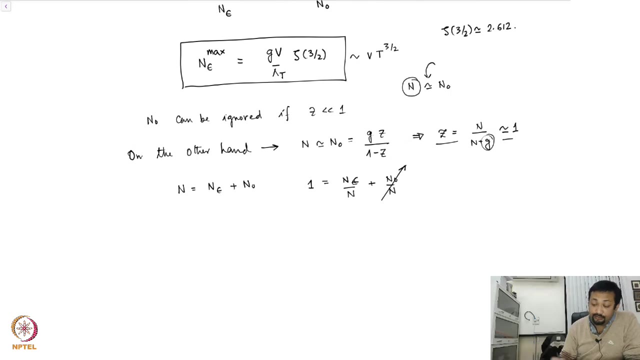 So basically, if n 0 is not sufficiently large so that you have not hit the z to 1 limit, then in the thermodynamic limit you can ignore this term and most of the particles are accommodated in the excited states. In contrast, whenever you have populated all, 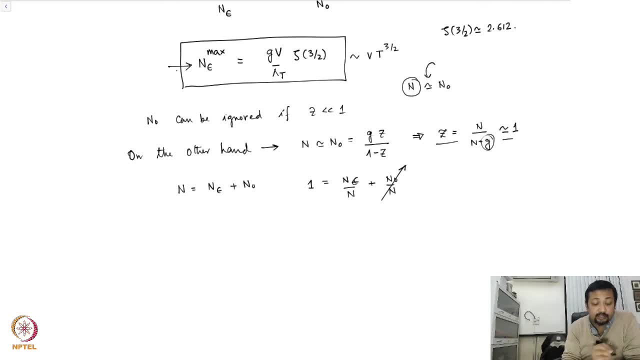 the excited levels. there is a limit, this epsilon max, you have reached. you start populating the ground state and that is when, If z is equal to 1 and n epsilon is equal to n epsilon max, then you have populated all your excited energy levels and then essentially n, 0 is given by. you have hit the limit of z. 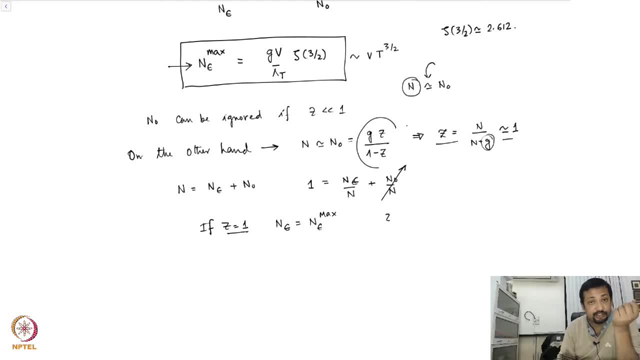 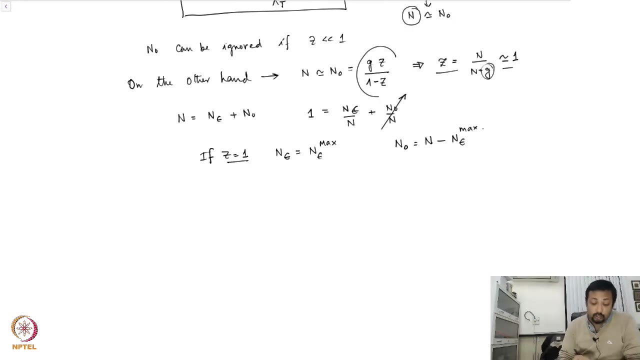 to 1, as z is equal to 1.. So you see, the n? 0 diverges. So, essentially, the number of particles in the ground states is given by total number of particles minus n epsilon max right. So we conclude therefore that n epsilon over n is equal to 1, for z less than 1 and 1 is 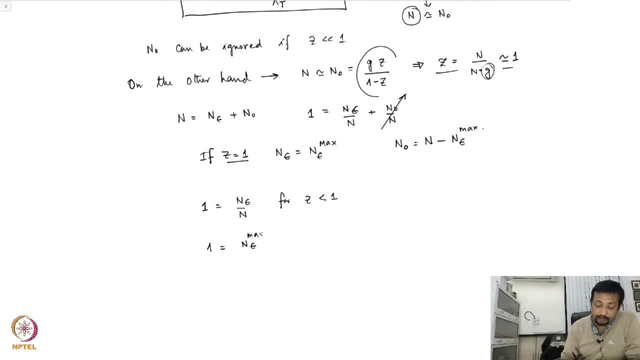 equal to n epsilon by over n plus n. 0 over n for z is equal to 1.. Therefore, we can see that when the total particle number is less than n, epsilon max, which is g v over lambda times zeta three half, or we can rewrite this condition as n lambda t over g v is less than. 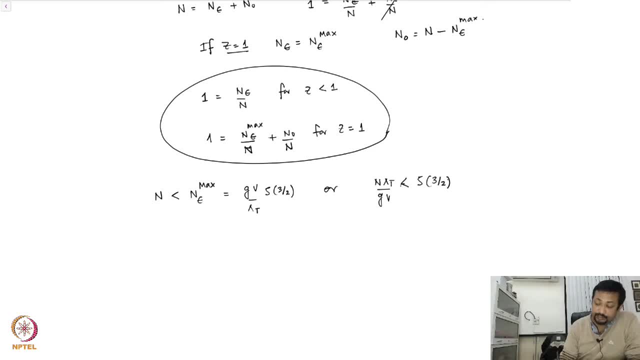 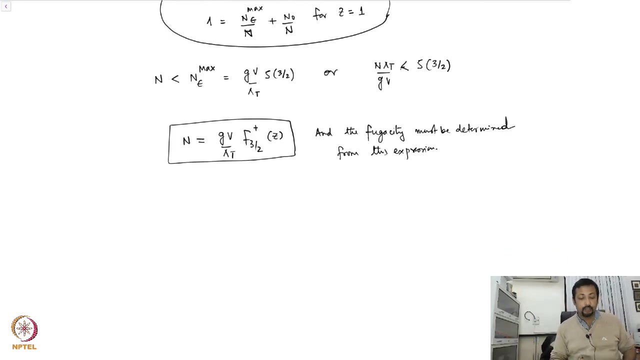 zeta of three half. That means you can still accommodate the particles in the excited levels, so that you have this expression, So n and the fugacity. the fugacity must be determined by the from this expression, as we have done it for a fermion system, for an ideal fermi gas. Now, 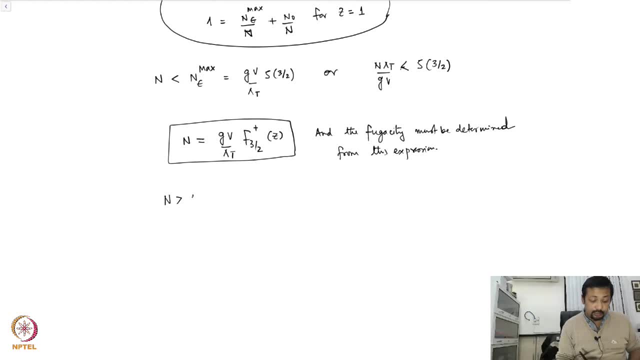 in contrast, when n is greater than n, epsilon max, which is less g v over lambda t zeta three half, or n lambda t over g v is greater than zeta of three half, then you have hit the limit in putting particles in the excited states. Therefore, in that case, your n 0 is given by: 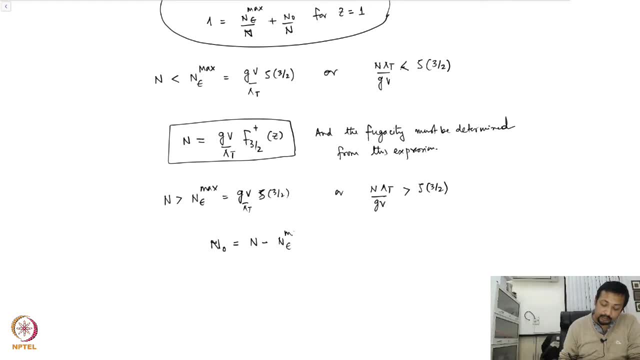 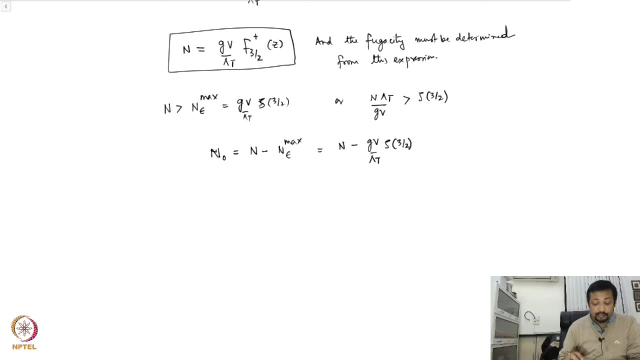 l minus n epsilon max, which is n minus zeta of three half. This means that there is a condition at which point the condensate can appear. I can figure out a temperature, So I can clearly see that, based on this, the condensate starts to appear. 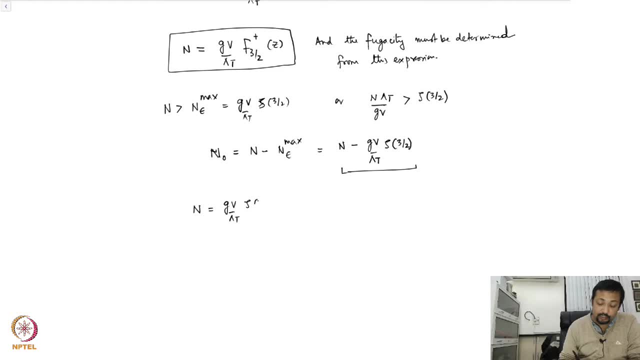 when n is g v over lambda t zeta to the power three half. That means that when you number of the particles in the system has hit the upper bound upper limit of n of the number of particles you can put in excited levels, The condition. 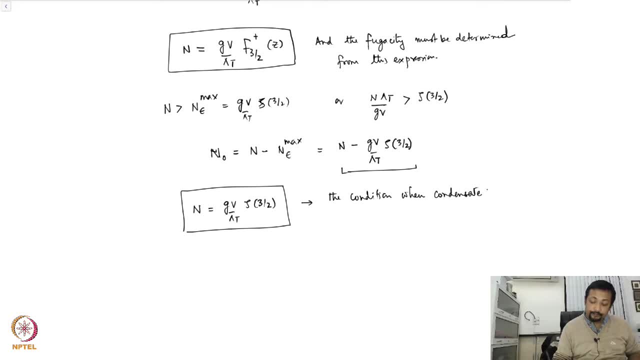 when condensate starts to appear again. at this point I would like to iterate that look, even though we are talking about a condensation, and whenever one talks about the condensation one talks about visualizes a condensation in the real space- it is not really a condensation in real 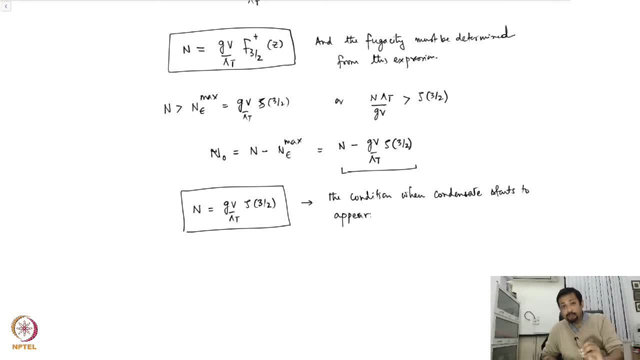 space. it's actually a condensation in a momentum space. all particles with whatever you've been talking about is labeled by this momentum vector k. the single particle levels are leveled by the momentum vector k. So what is actually happening is you are actually populating the 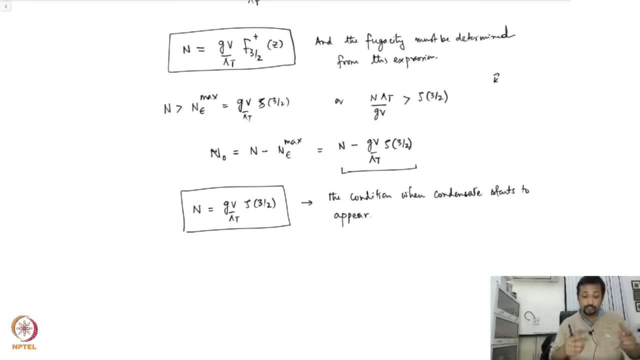 state with the 0 momentum, So it is a. if you can visualize the momentum space, then you are going to see a peak which is starting to appear in the 0 momentum state, and that is exactly what people have seen in experiments. So this effectively also means this essentially: 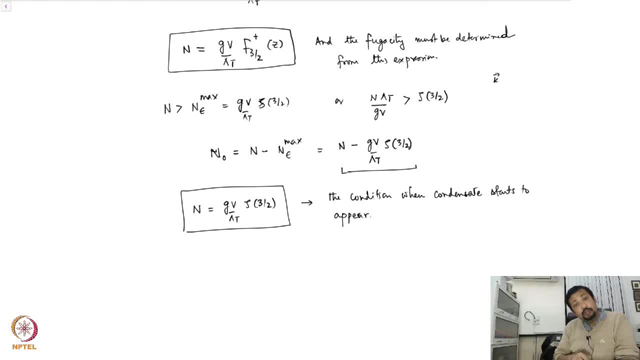 means That for large enough temperatures you have sufficiently large amount of thermal energy to excite the particles in the excited states, So that they are in the excited states, but as you keep on decreasing the temperature, as the temperature comes down- sorry, the density. 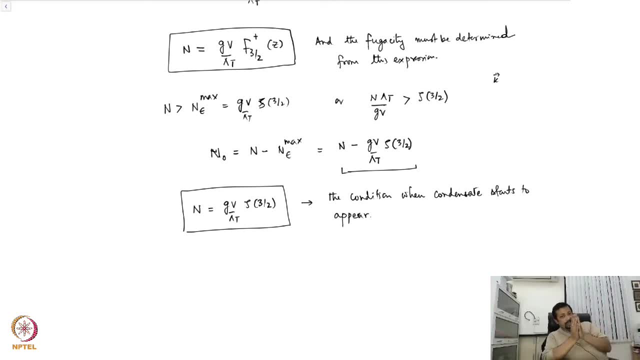 becomes high, or either you could have the temperature coming down, become smaller and smaller, or the density Is raised, which means you keep on adding particles and particles until you hit this criteria. what essentially happens is the positive correlation between the bosons ensures that they go, and 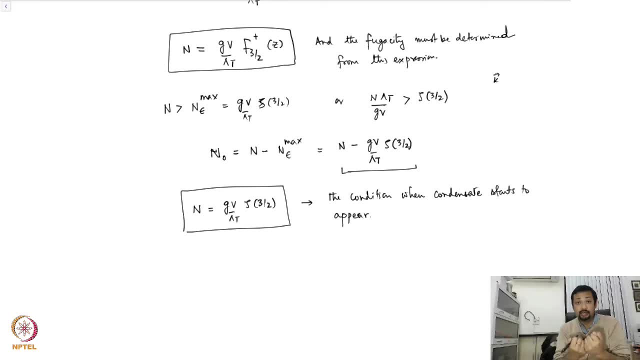 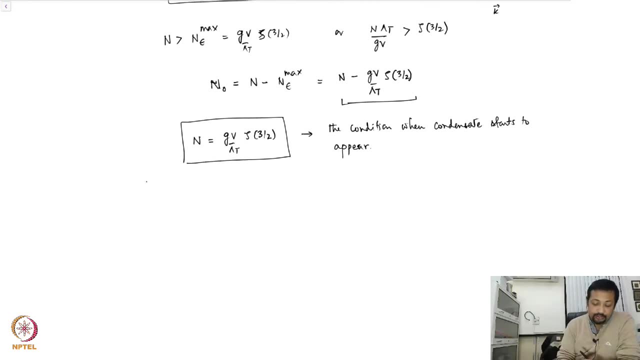 because they are attractive, So they go and sit at the ground. state energy epsilon equal to 0. So defining x equal to n, lambda t over g, v, then The fugacity Is defined by z is equal to 1.. 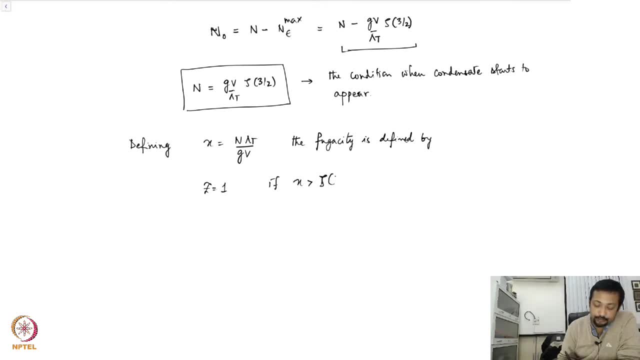 If x is greater than zeta of Three half And Solution Of x is equal to f plus three half z. So fugacity- Something is wrong here. Fugacity Is equal to 1 if x is greater than zeta three half. 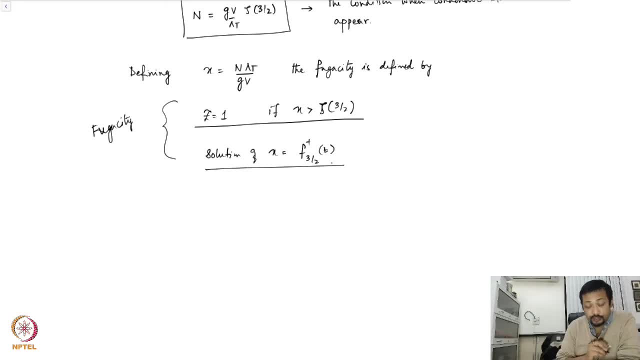 And or is the solution of this, When x is less than Zeta, two Zeta to the power Three half. Recall the first leading order. correction to this function: f three half Of Zed, F three half Goes. 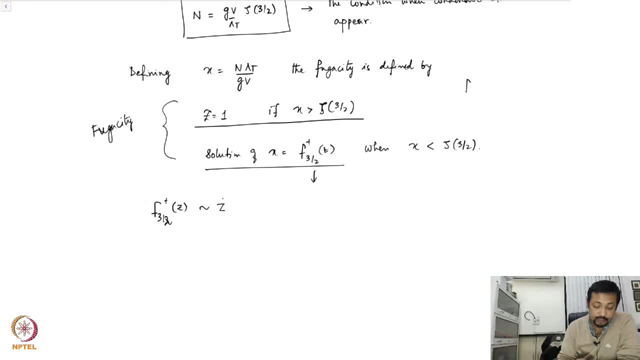 As Zed, For Small enough Zed, So that you have the solution x equal to Zed If you want to plot the fugacity, So that you have the solution x equal to zed If you want to plot the fugacity. 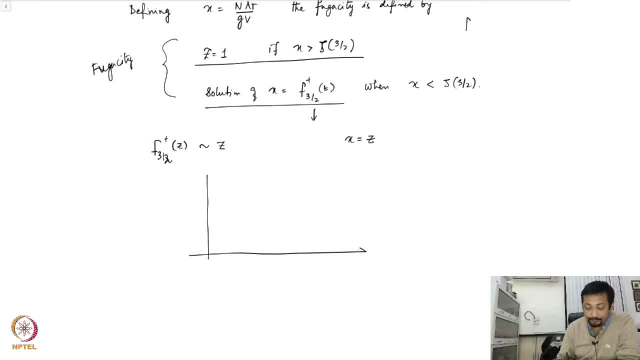 If you want to plot the fugacity. So this is the final solution. So this hits a value One Whenever Your x is greater than Zeta three half, But for small enough. So this hits a value. 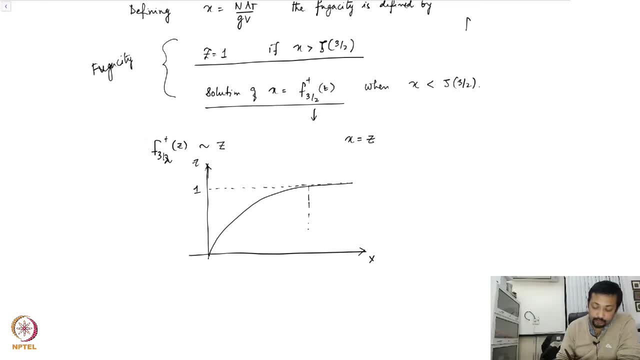 One. Whenever Your x is greater than Zeta three half, But for small enough Zeta three Half, You will have. z is equal to x, You will have. z is equal to x, Not really So the. 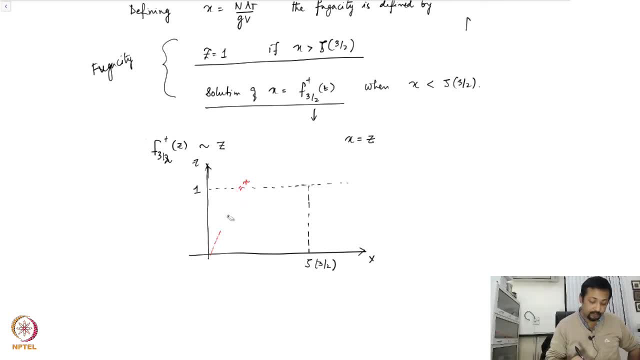 Not drawn to schematics, So let us just quickly draw it first, For small enough I am going to have, And you expect that the curve becomes Something like this way, So let us Shift it a little bit to the right. 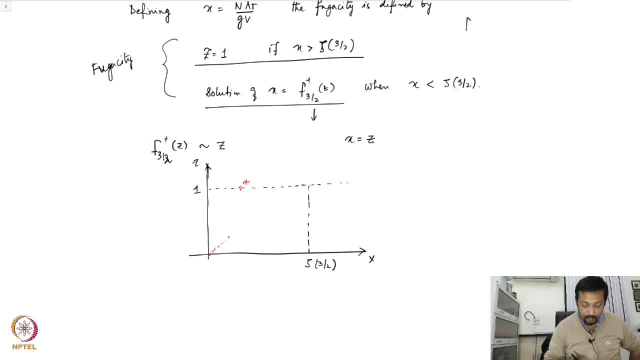 So that The Curve Becomes Something like this. So let us Shift it a little bit to the right So that Curve Becomes Something like this. So that Curve Becomes. 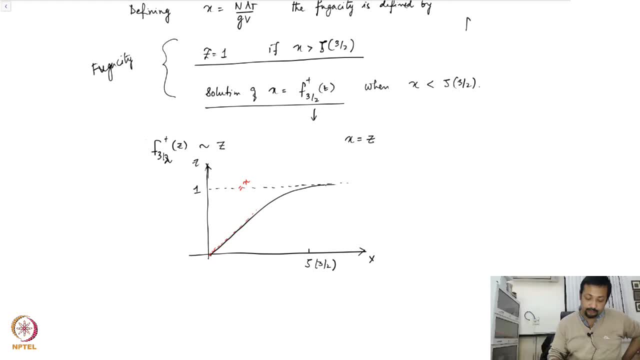 Something like this. So that Curve Becomes something like this. So let us Shift it to the right So that We can see that this Is going to be your zeta three half and not This. 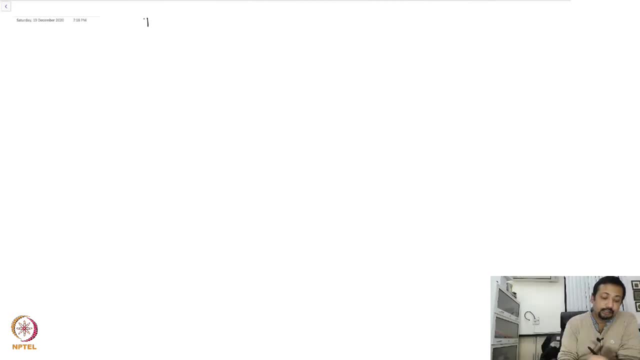 So this is how your curve should Look. The condition For condensation To appear Is given by equal to zeta 3 half. right, which is n, lambda t over gv is going to be zeta of 3 half. so now 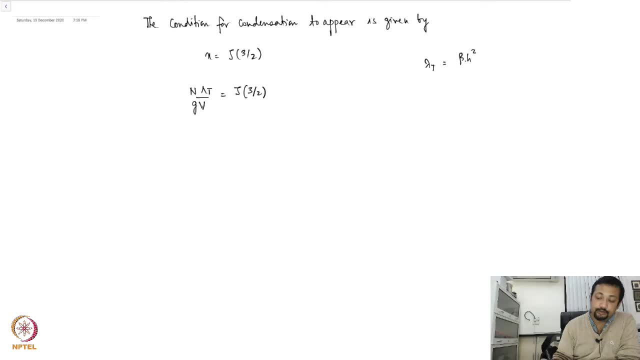 lambda t is beta h squared over 2 m pi raised to the power half, so that the thermal de Broglie volume is beta h squared over 2 m pi raised to the power 3 half. so then n over gv, 1 over zeta 3 half, is equal to 1 by beta h square. 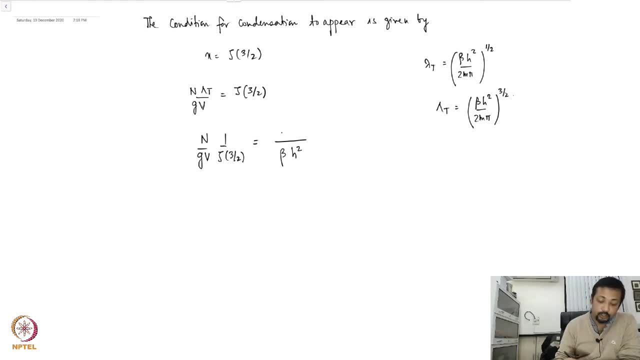 twice zeta 3 half m pi raised to the power 3 half. so capital N by V is a small n, the number density g, zeta 3 half raised to the power 2. 3rd, I have 1 over twice m pi, which is going to be your k B. 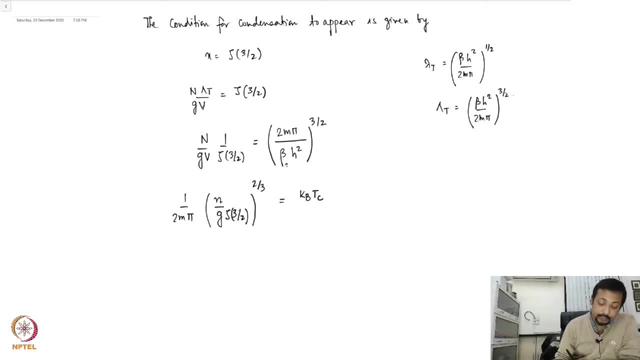 DC, so it will replace the beta here by beta C, indicating that this gives me the temperature. so you have a critical temperature K B of DC which is given by one over 2 m pi and over G times. zeta of three, half raised to the power times, the. 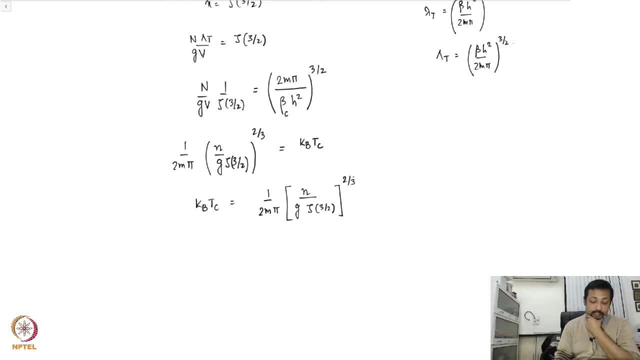 2 by 3.. I am missing out a factor of h square, so that this has to be h square in the denominator. So this is the critical temperature that you are looking at. At this temperature your condensation starts to happen and you start to see a condenser that appears at the k equal. 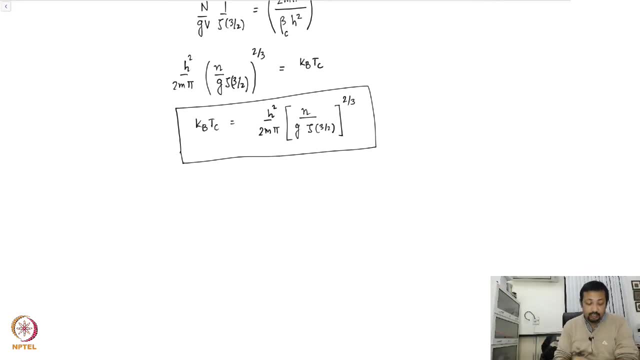 to 0 momentum state. Now the particle number in the excited state n epsilon over n is equal to 1 for T greater than T c, because all the particles that you put in essentially goes into the excited states If you are away from this critical temperature. 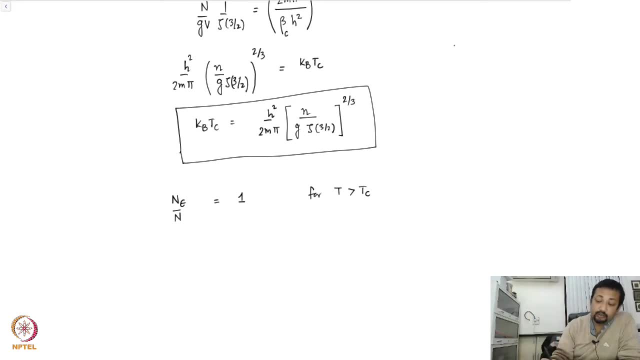 occurs. but the moment you hit the critical temperature, you essentially hit a limit of g v over lambda T, zeta 3 half, so that this n epsilon goes as T to the power v, T to the power 3 half. And you clearly see that from this condition that we had, that this gives. 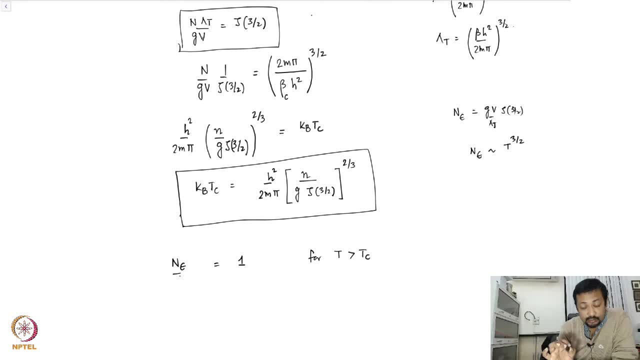 me the temperature At which the condenser starts to appear. so I can sort of write down this as: lambda T c, g v is equal to zeta 3 half, so that lambda T c is equal to g v over n zeta 3 half, right. 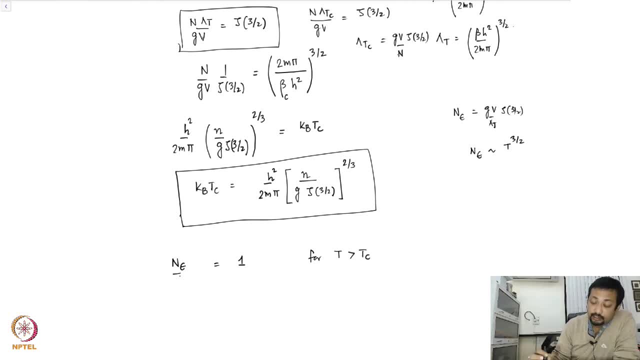 Or essentially I can write down g v over n And if I look over here then g v over n is equal to g v over lambda T, zeta of 3 half times zeta 3, half divided by n, which 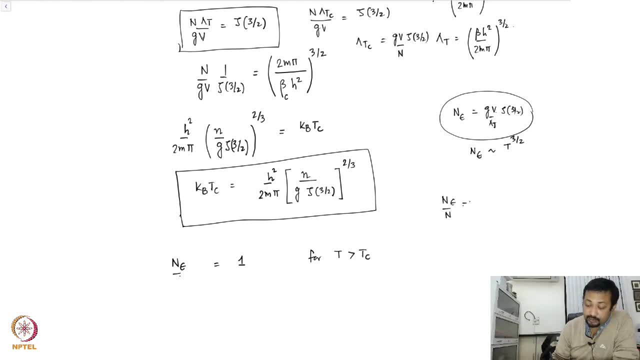 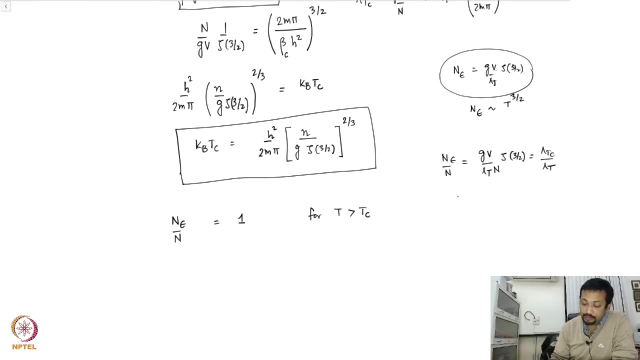 is n, epsilon over n is g, v, lambda T, n. zeta of 3 half, which is essentially lambda T, c over lambda T. So this is therefore Zeta 3 half, So Zeta 3 half, T over Tc raised to the power 3 half. So this is T over Tc raised to the power 3 half for T. 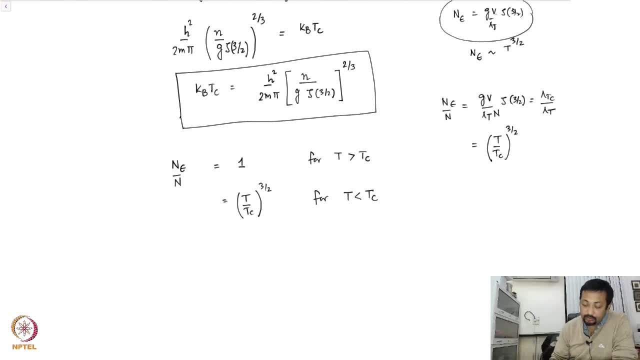 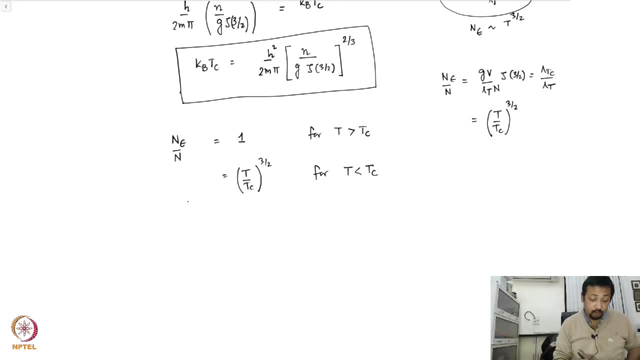 less than Tc. So as you start hitting the critical temperature you start to get this. Now the number of particles in the ground state is 0 for T greater than Tc. However, as you cross the critical temperature then this becomes 1 minus T over Tc raised to the. 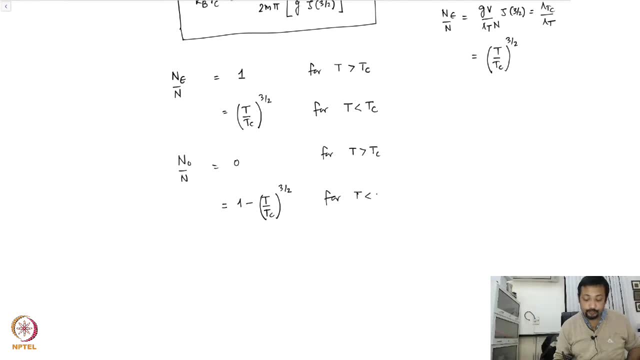 power 3 by 2.. And this expression follows from the fact that 1 plus Tc raised to the power 3 half, So this is T over Tc raised to the power 3 half. 1 is equal to n epsilon by n plus n 0 over n, So that n 0 over n is 1 minus n epsilon. 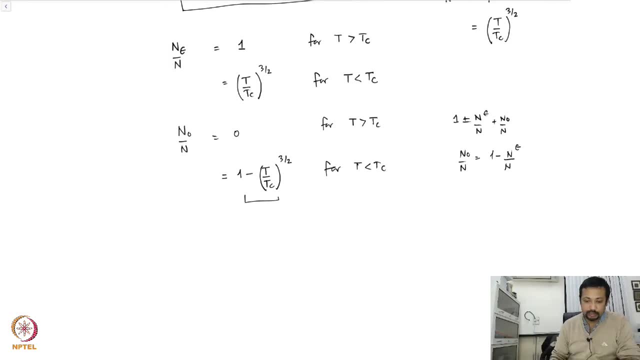 over n. If you carefully study these two expressions, one can plot them also. You see that as you approach 0 and 0 temperature, the number of this thing vanishes, so that I have T over Tc raised to the power 3 half. What does this result in? There is a reading about. 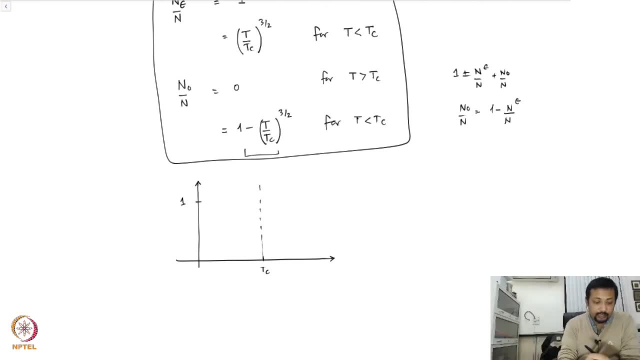 Tc, which is 1.. Then this is my Tc. Let us say we will draw a vertical line and this is 1.. Then this is going to be n epsilon over n number particles in the excited state. for T greater than Tc, Then this goes as this: And then, if T equal to n epsilon by n. So this is 1 plus Tc raised to the power 3 half. If you carefully study these two expressions, you will see that this is 1 minus Tc raised to the power 3 half. So this is 1 plus Tc raised. to the power 3 half minus n epsilon by n plus n, 0 over n, This is 1 plus Tc raised to the power 2 half. So you can see that this is 1 plus Tc raised to the power 3 half. So if you carefully,